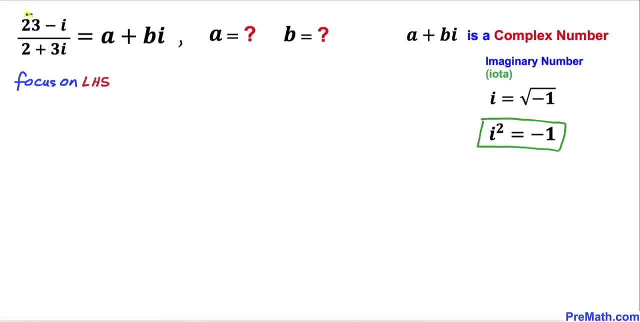 started with the solution, and here's our very first step. Let's focus on the left hand side of this equation, And here i have copied it down, and now we are going to rationalize this denominator part. Therefore, let's talk about the complex conjugates of this: 2 plus 3i. 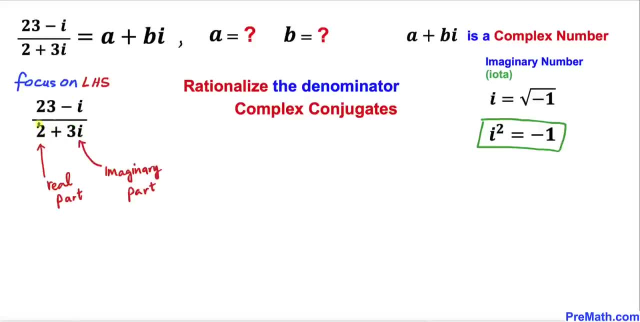 And before we go any further, just keep in your mind that this 2 is called real part and the part that has i with it is called imaginary part. Just keep in your mind. So the conjugate of this number, 2 plus 3i, is going to be simply 2 minus 3i, So we are going to multiply. 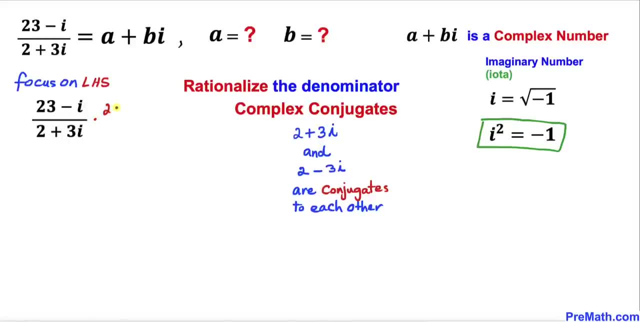 and divide by its conjugate. So I'm going to multiply by 2 minus 3i and divided by 2 minus 3i as well. And now let's go ahead and multiply these complex numbers on the top, and likewise I am going to multiply. 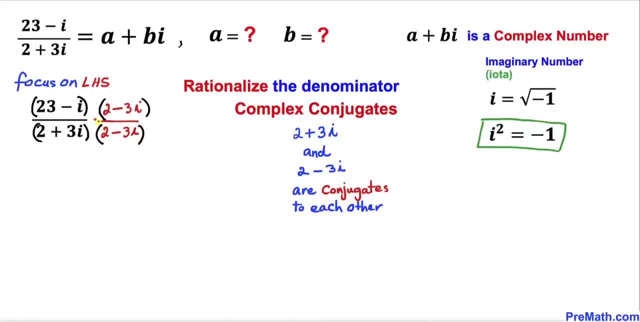 complex numbers at the bottom as well. so let's go ahead and multiply the top numbers by using this double distribution. so that is going to give us 46 minus 69 i minus 2, i, and then plus 3 i square divided. by now we are going to multiply these two factors. let's recall this identity. 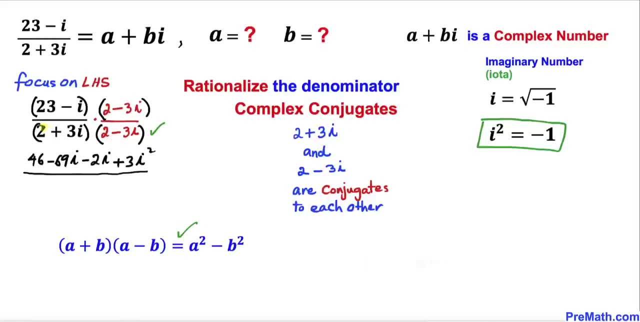 a plus b times a minus b, we are going to apply on this denominator, so the denominator could be written as: 2 square minus 3- i whole square. and now let's focus on this denominator part. and we are going to multiply this by 2 square minus 3- i whole square. and now let's focus on. 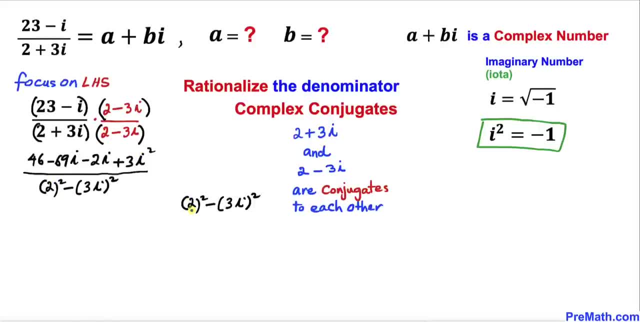 i have copied it down over here and now let's simplify this thing: 2 square is same as 4 minus. this is going to give us 9 i square, but we know that i square is always equal to negative 1, so wherever we see i square, i am going to replace it by negative 1, so therefore we can write this: 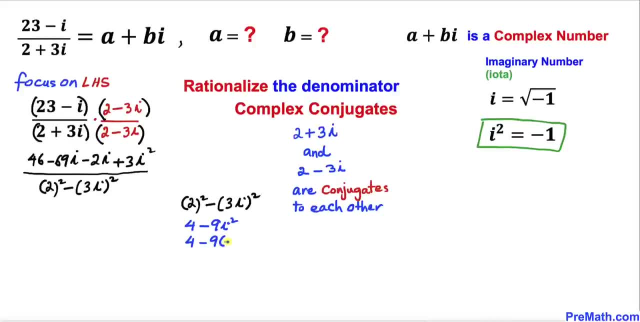 thing as 4 minus 9 times negative 1, so that is going to give us 13. so, therefore, i am going to replace this whole denominator part by 13, and now let's focus on this numerator and let's focus on this: i square, and we know that i square is always equal to. 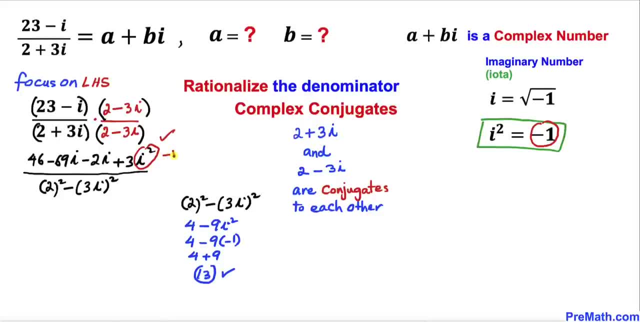 negative 1. so therefore i am going to replace this one by negative 1, so the numerator could be written as 46 minus 69, i minus 2, i then plus 3 times negative 1 divided by. i am going to replace this denominator by this 13, so i'm going 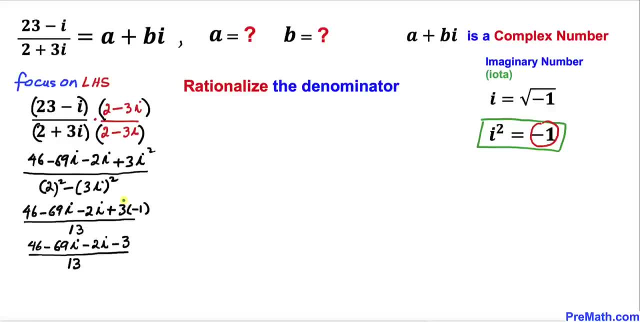 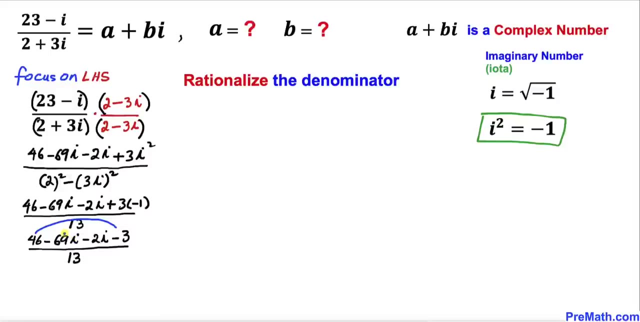 to just write down 13 and in this next step i just replace this 3 times: negative 1 is going to become negative 3 and the rest are same. and now let's go ahead and combine the like terms. i'm going to write down 46 minus 3 and then negative 16. and then i'm going to write down 46 minus 3 and then 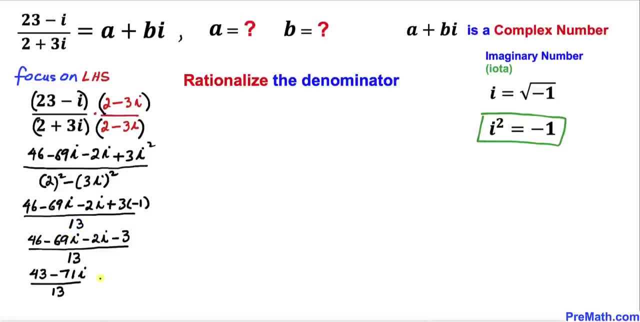 i'm going to write down 49 i minus 2. i now let's go ahead and break down these fractions. i can write this one: 43 divided by 13, and then minus 71, i divided by 13, and in this next step, this part, 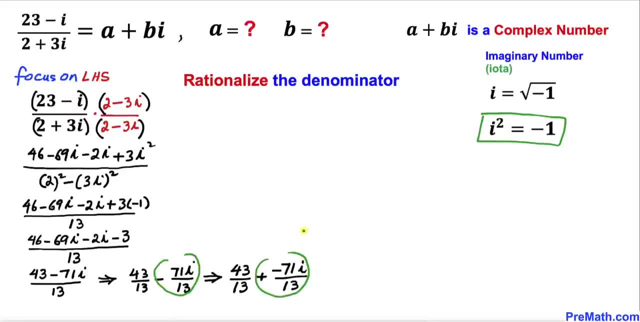 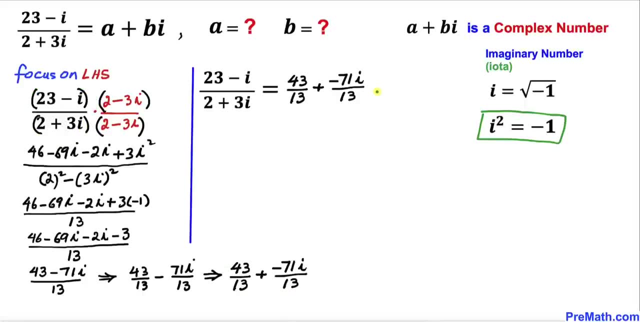 could be written as like this one. so therefore this left hand side has turned out to be equal to this one, so therefore we can equate them, as you can see over here. but we also know that this left hand side equals to a plus bi, as you can see in this original question. now let's go ahead and 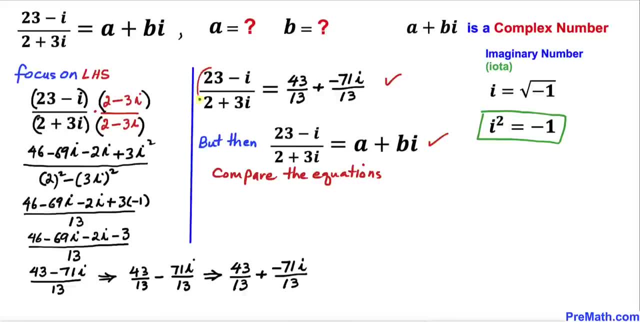 compare these two equations. we know that the left hand sides are same, so the right hand sides have got to be same, and now we can see that this part corresponds to a and this part, negative. 71 divided by 13 corresponds to b. so therefore this part is our a. 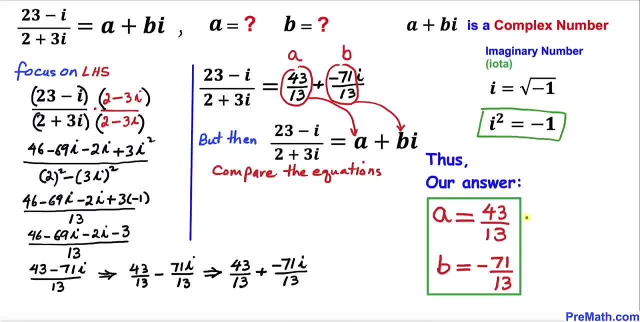 and this part is our b. so thus our a value turns out to be 43 divided by 13, and b value is negative 71 divided by 13.. thanks for watching and please don't forget to subscribe to my channel for more exciting videos. bye. you. 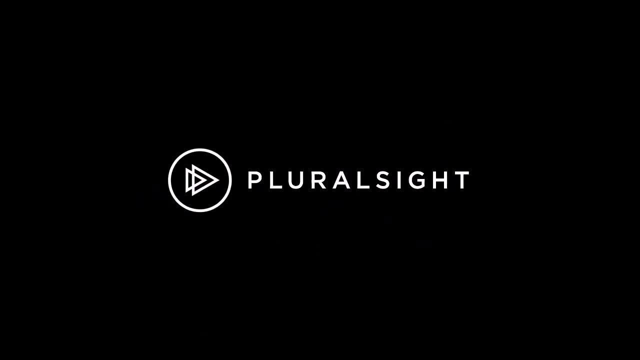 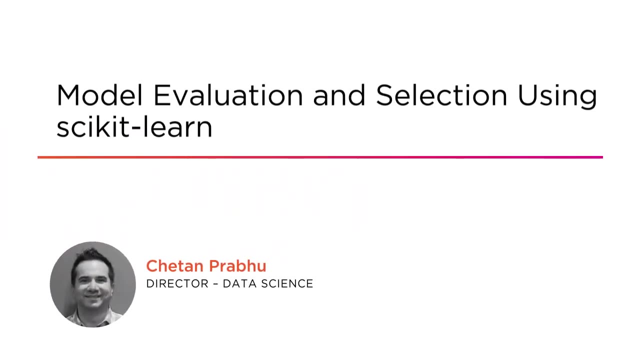 Hi everyone, my name is Chetan Prabhu and welcome to my course: Model Evaluation and Selection using Scikit-Learn. I am a data science practitioner and leader with over 10 years of data science experience in industry. In this course, we're going to learn about techniques and methods. 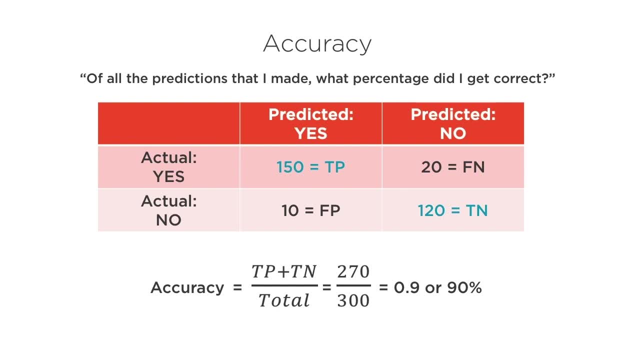 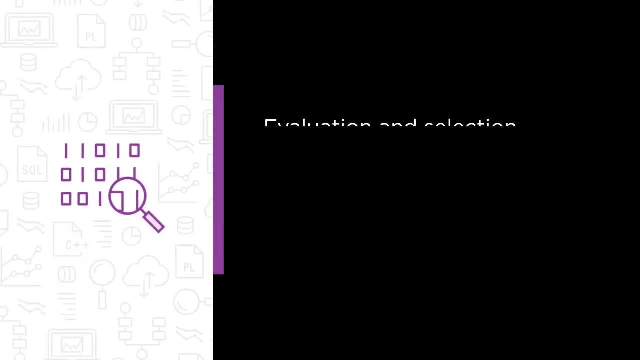 that you can use to evaluate how well your machine learning model is performing, and also how to select the best model from a set of models that you've built. Some of the major topics that we'll cover include why model evaluation and selection is important, and useful metrics and formulas. 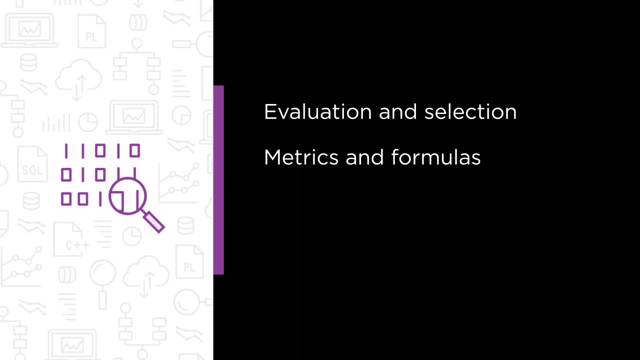 used to measure the performance of classification and regression models separately. methodologies to perform model selection: avoid overfitting and picking the model that will perform best in the future. Finally, you will learn how you can implement all of these ideas in Scikit-Learn. 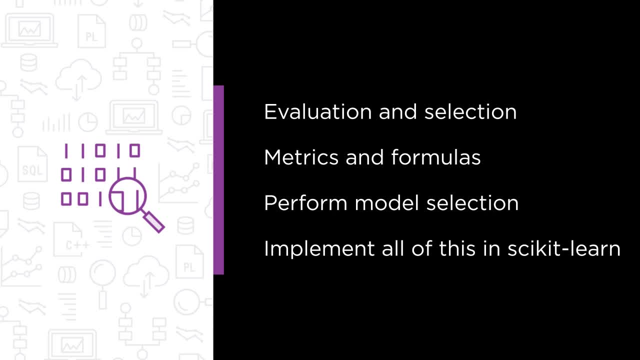 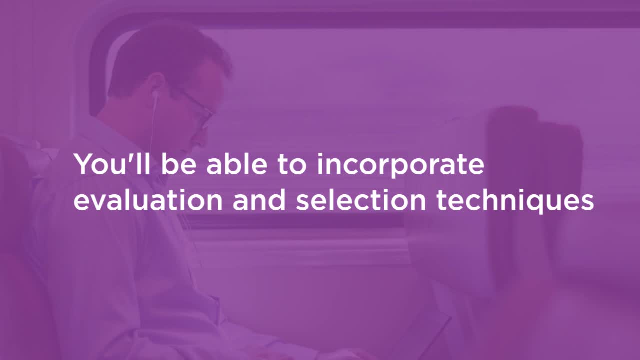 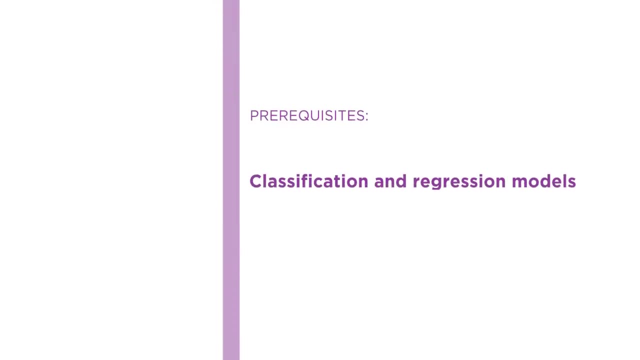 which is a major machine learning library in Python. By the end of this course, you'll be able to incorporate modern evaluation and selection techniques within your machine learning workflow, all powered through Scikit-Learn. But before beginning this course, you should familiarize yourself with how classification 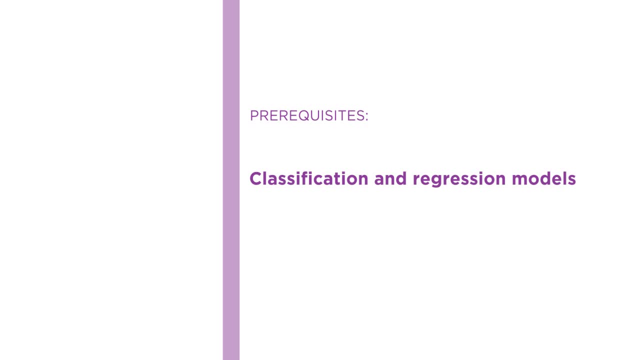 and regression machine learning models are built. I will assume you're comfortable with what a machine learning model is and how they are created. I hope you'll join me on this journey to learn more about improving your machine learning workflow with the Model Selection and Evaluation. 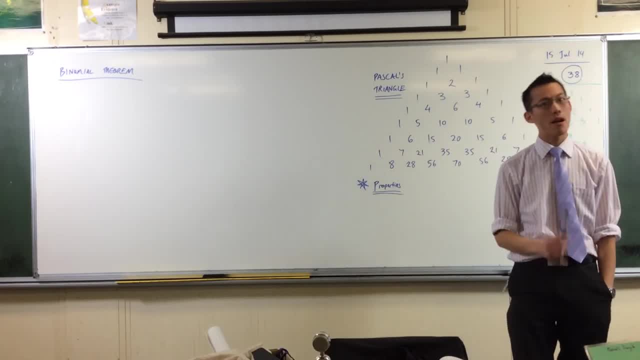 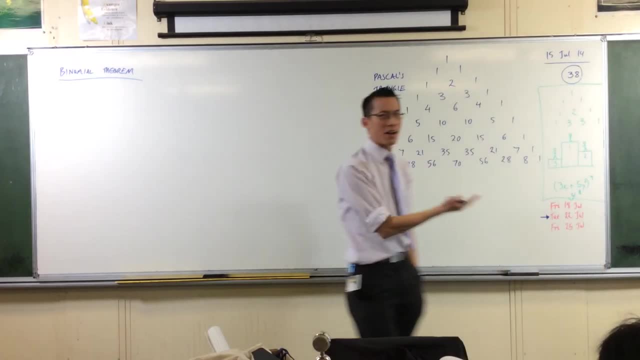 Pascal's triangle has a whole bunch of properties, Very, very interesting properties, Far more than I'm going to talk about briefly today. By the way, it's worth noting, Pascal was not the guy who invented this triangle. He's not even the first guy to have spotted the pattern.